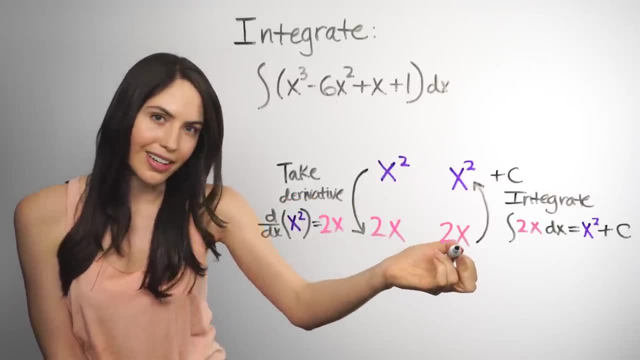 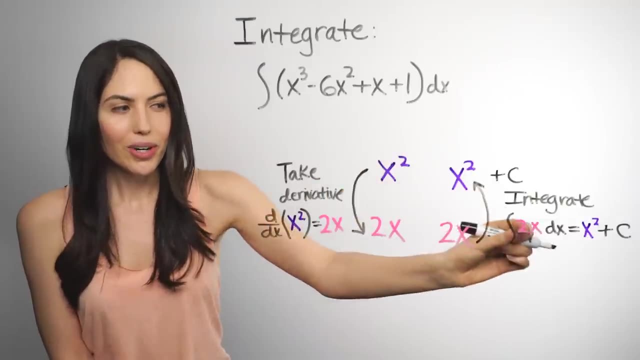 we differentiated, then integrating it will be getting back the original function to get back our original function, and the derivative will be getting back our original function, So up. So what we're integrating is the derivative of some other function that we will find. 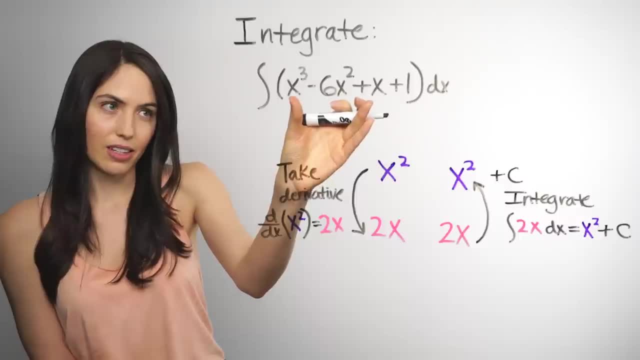 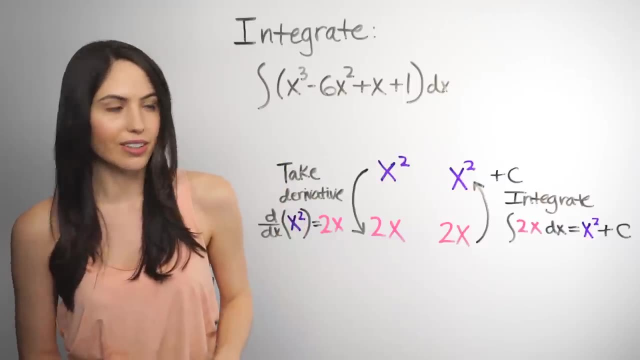 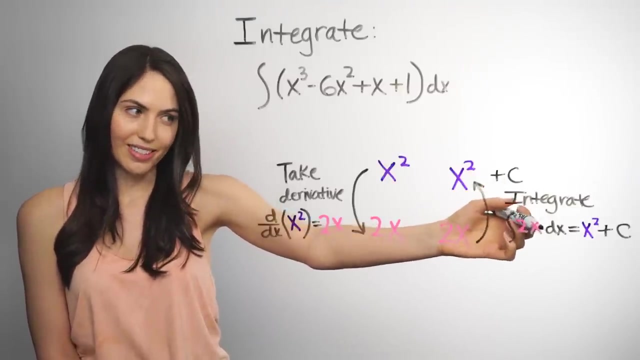 So even here, what we're integrating is the derivative of some other function that we will find, and that's the antiderivative or indefinite integral. integral, This reads as the integral of 2x with respect to x, or antiderivative 2x with respect to x, The dx. 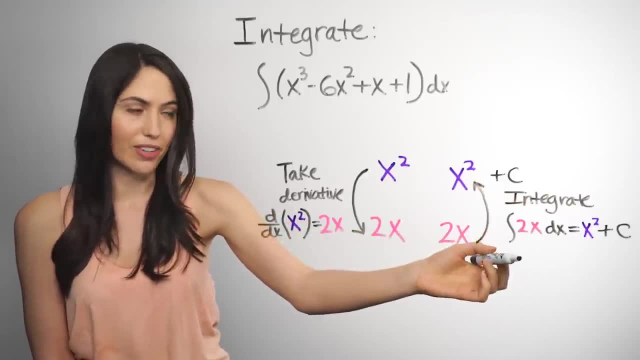 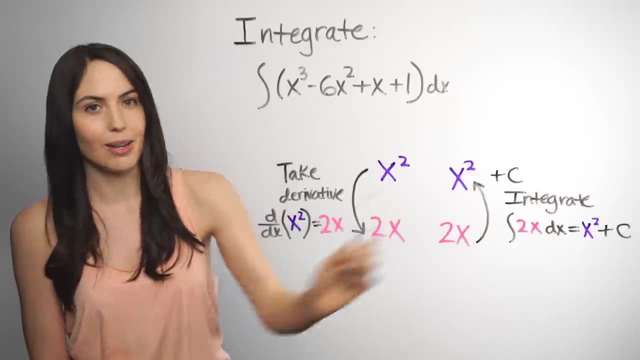 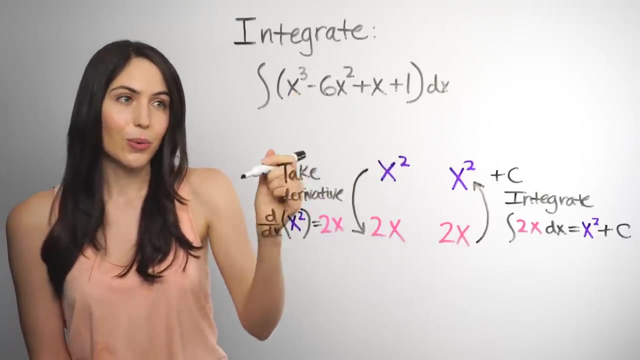 differential just tells us that x is our variable of integration, that we're integrating with respect to x and not some other variable. And I will explain the plus c in a bit. So for a polynomial like this, with a bunch of terms added and subtracted, we can integrate. 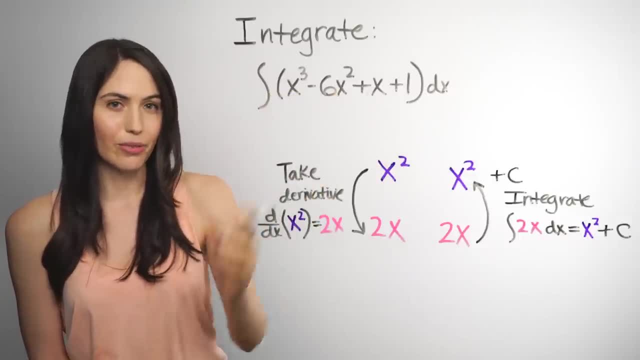 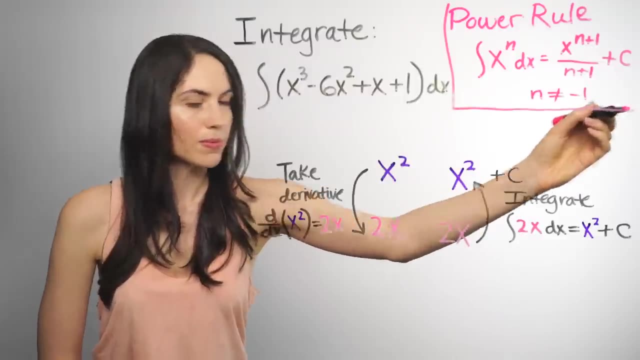 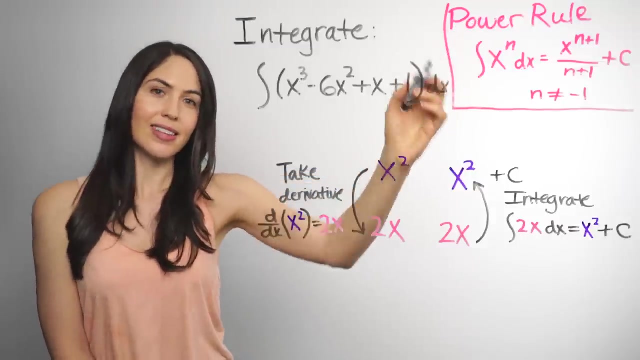 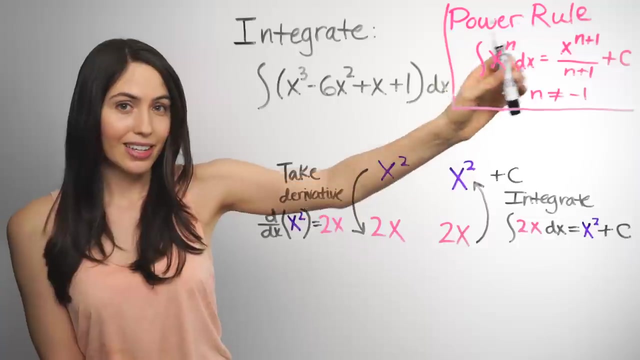 each term one by one and then string them together for the full integral. So let's do it. So this first term is an x power, so we can use the power rule And all that says is that if your power is not negative, 1, if it's any other power, the integral of x to the power. 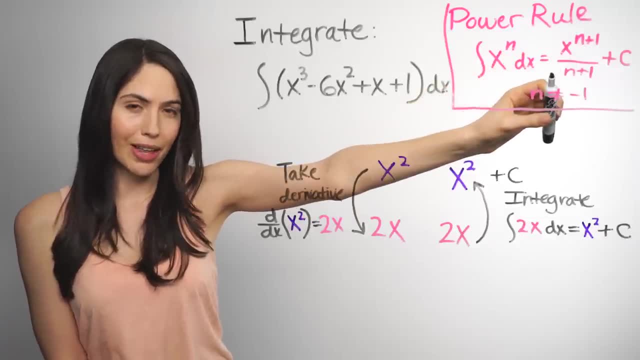 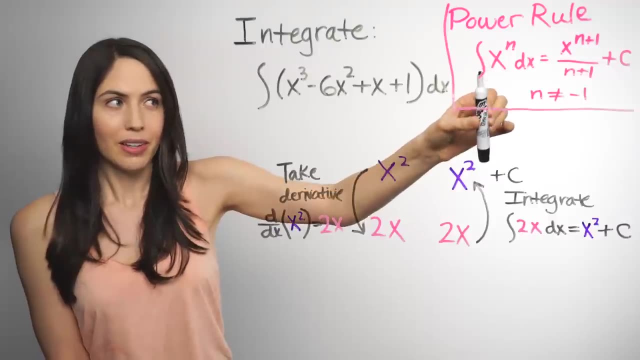 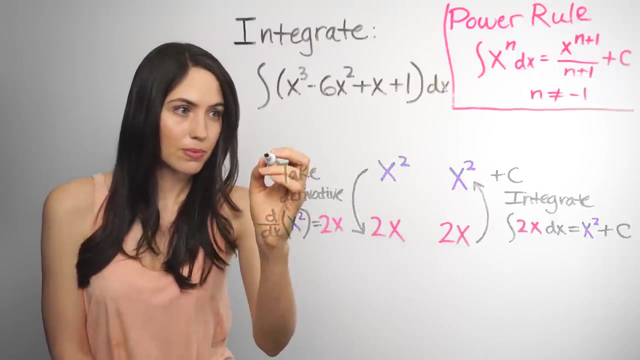 is x to the power raised by 1, over that power raised by 1, plus c. So for x to the third power, the integral is: instead of x to the third, it's x to the fourth over 4.. 1 and 2 is negative, 1 minus 1.. If you have an x, then you don't have an x squared. 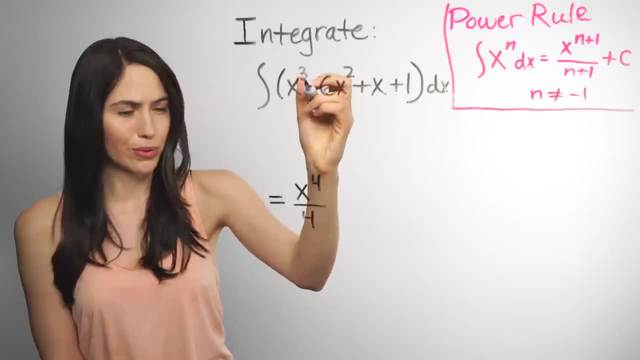 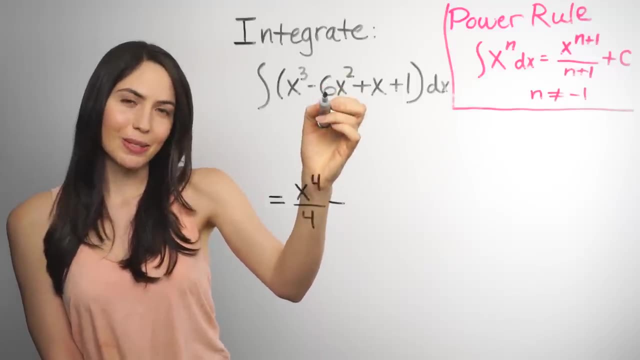 because it's 0.. So I take x squared and I leave it at that time. in conclusion, So this one, if I was to spend it on anything else this time, or this side or that side, and then put it back in to look for the 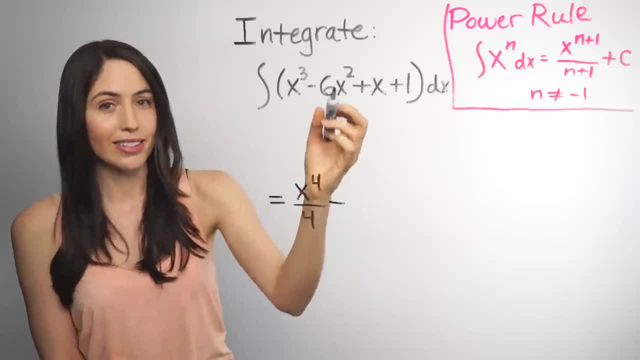 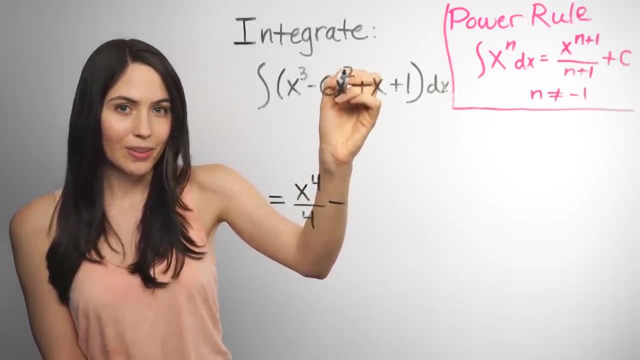 persona here, whereas the your powerften switch it back, because this side needs some wealth, it needs power. Now, with this part, this fundamental sum, itっと they're reference Americans. it'll be, because that's what it says in the brighten sum we're working on. And that table will detail that, And we don't need to do anything further to prove any of this, Because this is probably just a brief couchshow. I don't know about any other stuff. no internet libraries that are as simple, but why not? One of the reasons why we need a hyper teams. 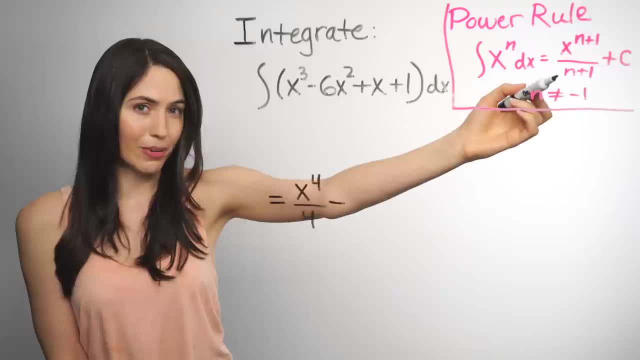 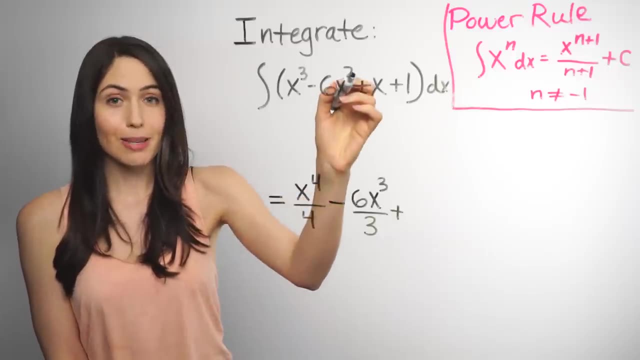 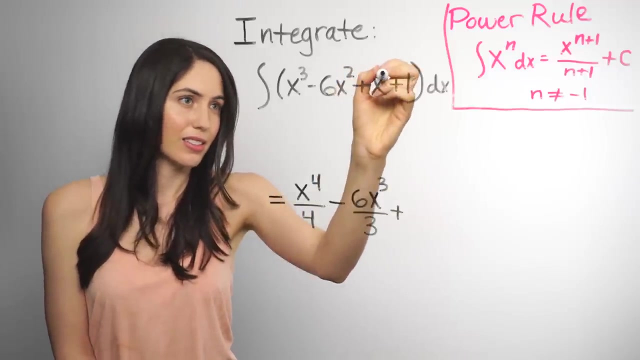 second power, it's going to be x to the third divided by 3, and we'll clean that up later. We can also keep the addition, so the sum and difference rules. What about x? Well, that is a power of x. There is this implied one or understood power. 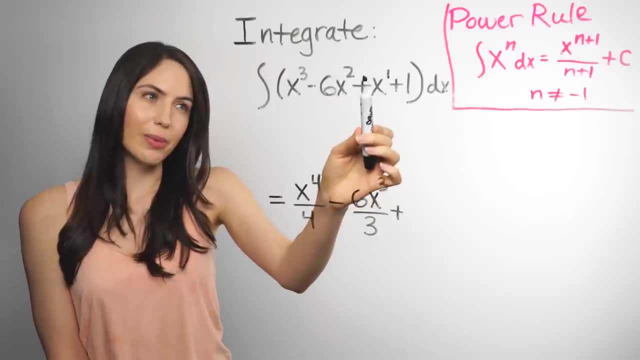 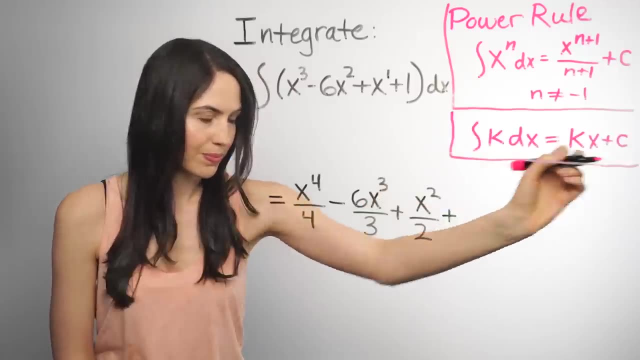 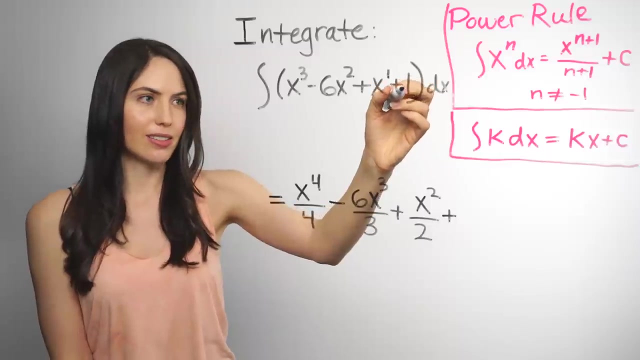 of one. so if we use the power rule on x to the first power, it becomes x squared over 2. And any time you have just a constant term, the integral of that will just be the number times x. so the integral of one is one times x or just x. 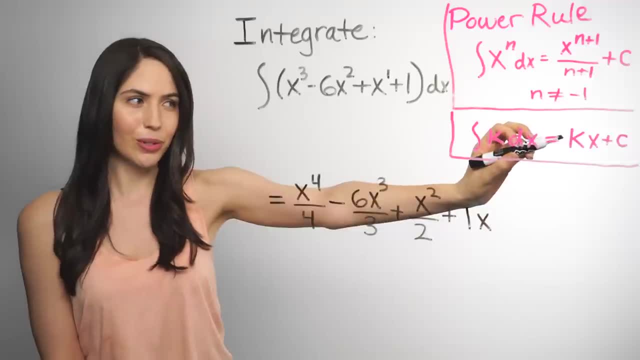 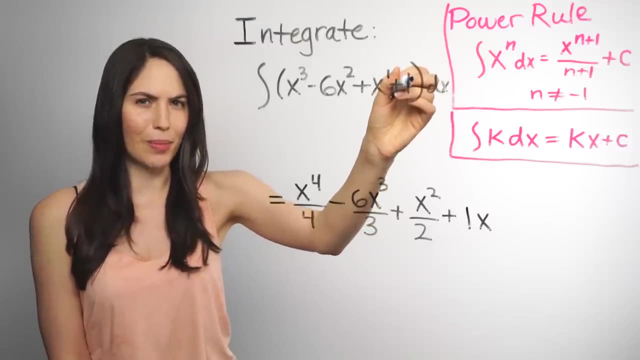 And some people think of this as a separate rule, the constant rule, and other people think of it as the power rule. There is technically an invisible x to the zero power here. So if you use the power rule on x to the zero, you get x to the one over one. 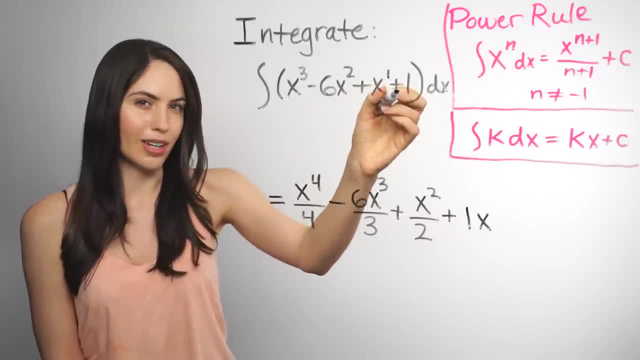 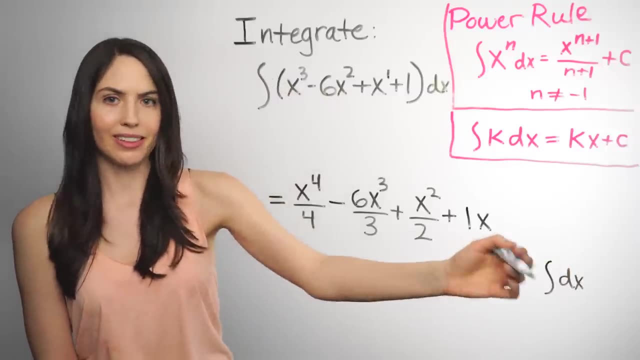 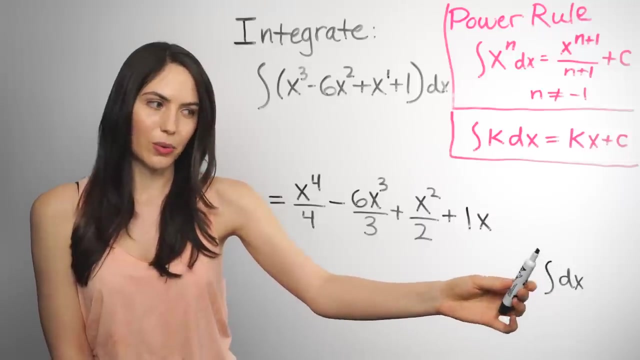 Any way you look at it, the integral of one is one times x or x, And, by the way, if you ever saw something like this, there is an implied one there. so that is also the constant rule. The integral of this would just be x, And at this point you may have a little bit. 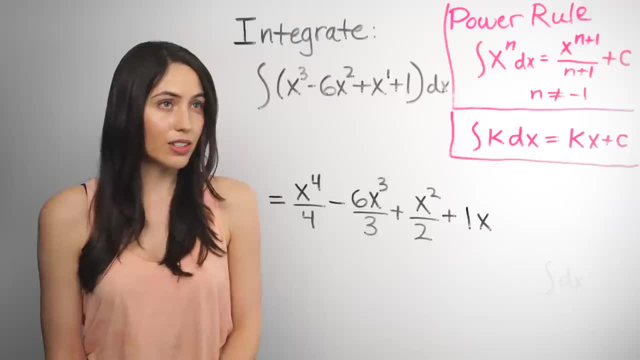 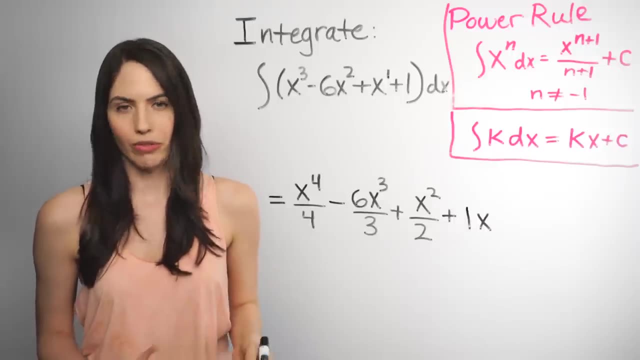 of deja vu. So what you can do with some of these rules. a lot of these integration rules seem vaguely similar, but opposite to derivative rules, And you can pretty much reverse a lot of derivative rules and get the integration rules. but not all of them are similar and have a counterpart. 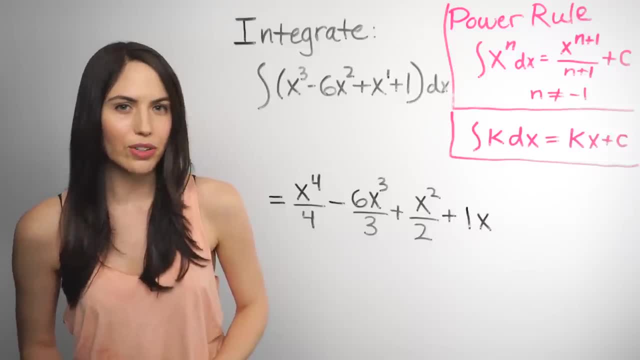 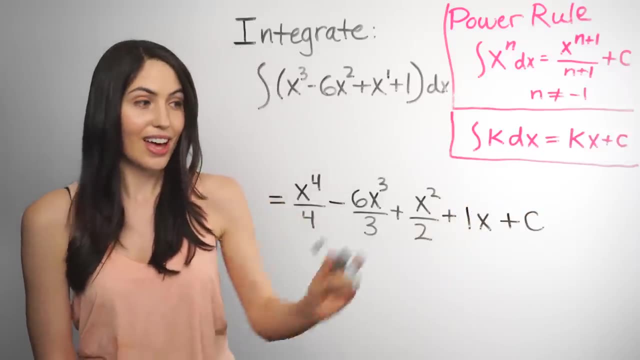 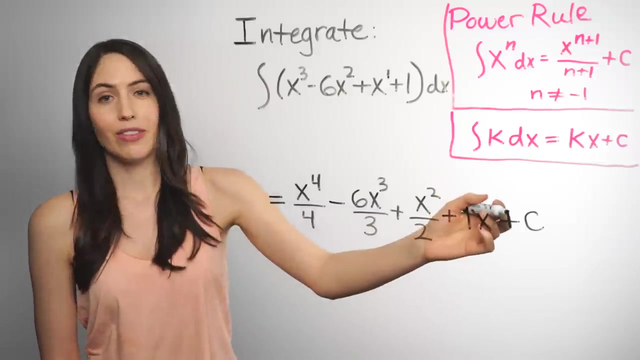 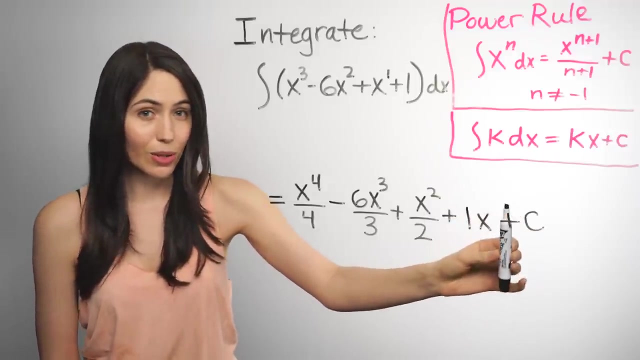 like there is no product rule or quotient rule for integration, And we are not done. We have to add a constant plus c at the very end, And this is important Because we don't know if there was a number there originally and, if so, what it was. So we put this plus c as a placeholder and it represents all possible. 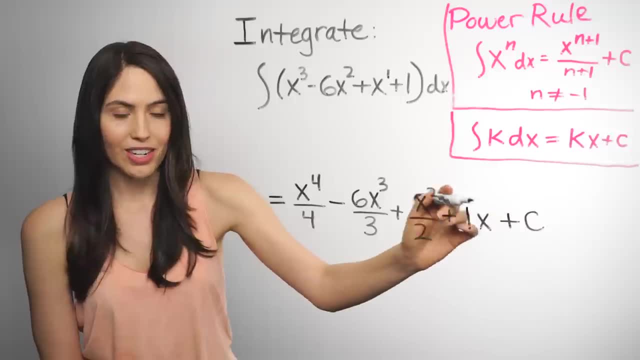 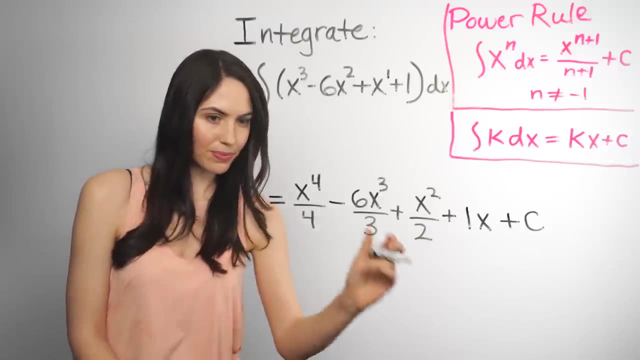 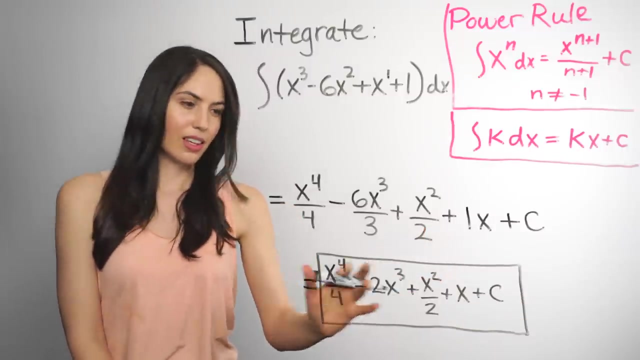 antiderivatives. You put that there just in case there was a number there like plus two minus two minus ten, whatever it was. Someone wrote to me how smart, as always, So here it is all cleaned up. Remember, this is the original function. higher level function. 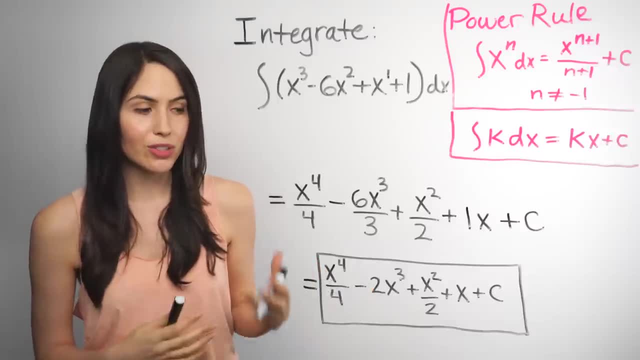 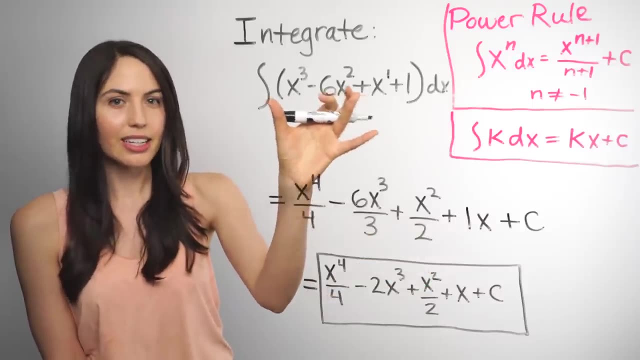 we got by integrating. So, if you want, you can check this answer by taking the derivative of it and you will get back your original integrand even though there's this plus c here, because, remember, the derivative of a constant is just 0.. 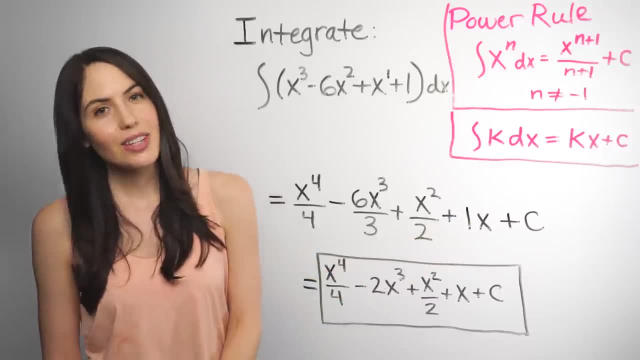 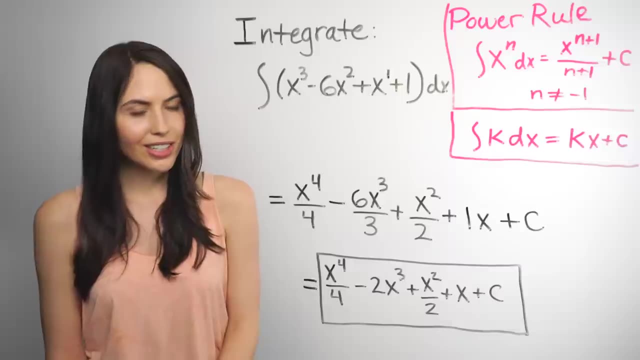 So that goes away. And in case you were wondering why I didn't put a plus c on every term as we went along integrating. it's a good question, It's just because it doesn't matter in the end. Like we could have done that, but in the end we'd. 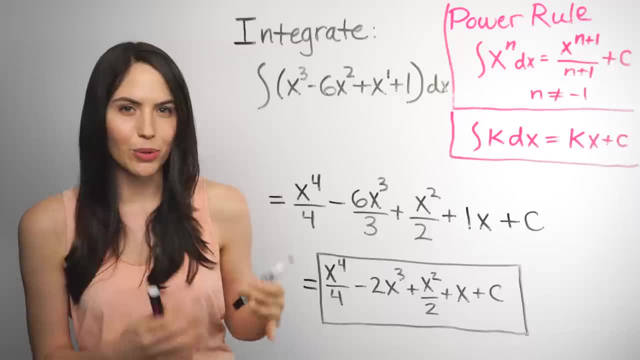 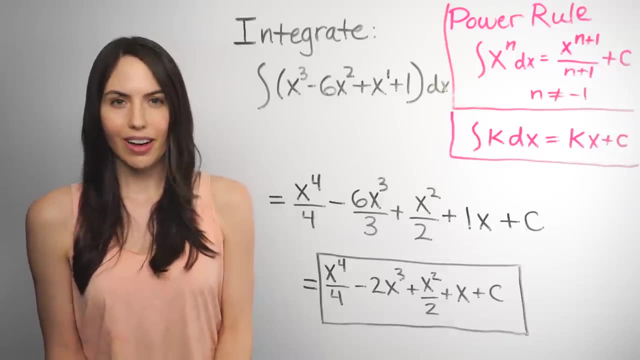 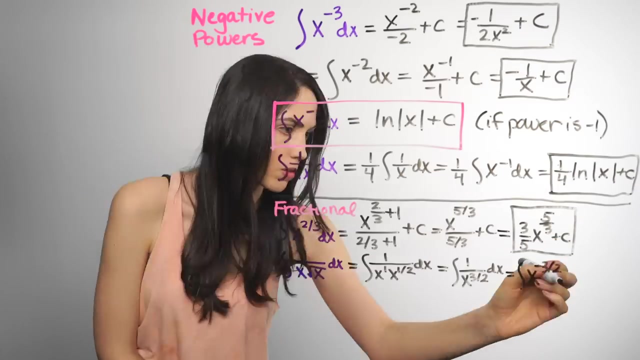 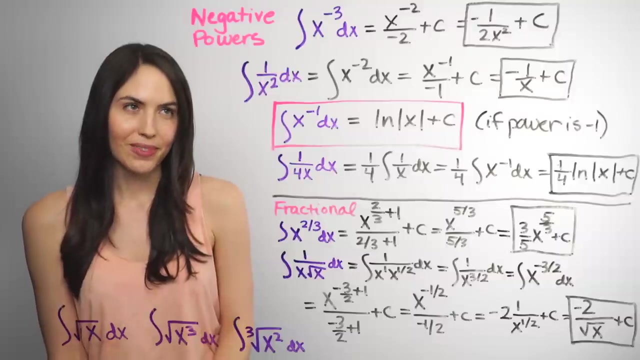 still have all these constants that add up to one constant? we still don't know, and we can still call that plus c in the end. So what about other kinds of powers? Maybe you knew it wouldn't always be so simple. What if you have a negative power? 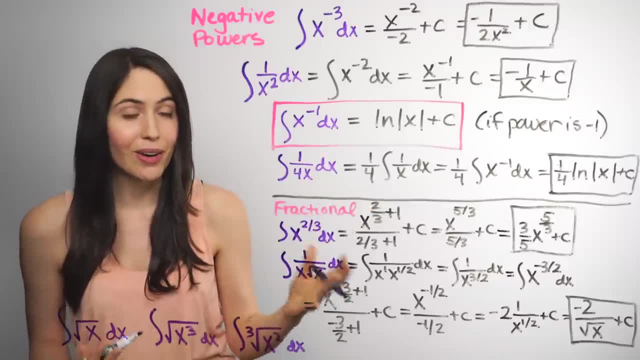 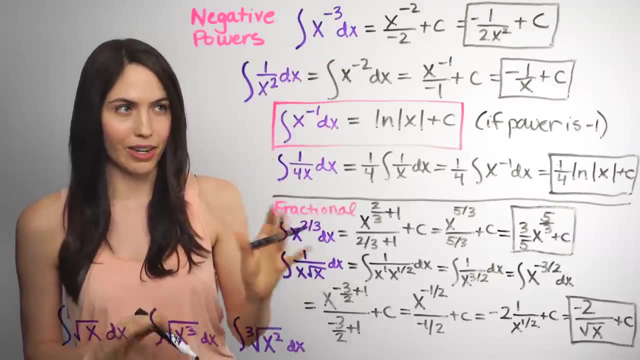 or a fractional power, or a negative fractional power, or a root. If you have a negative power, you can still use the power rule as long as your power is not negative 1.. So here this negative 3 power becomes negative 2 with the power rule. 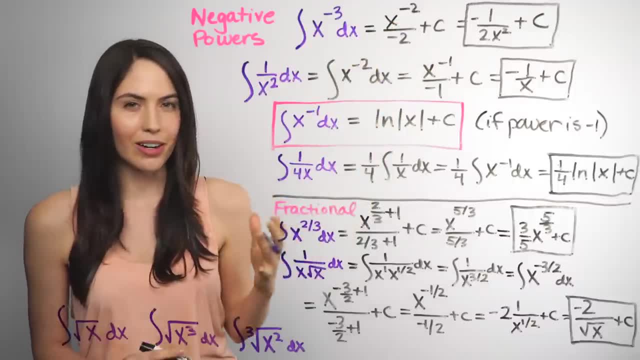 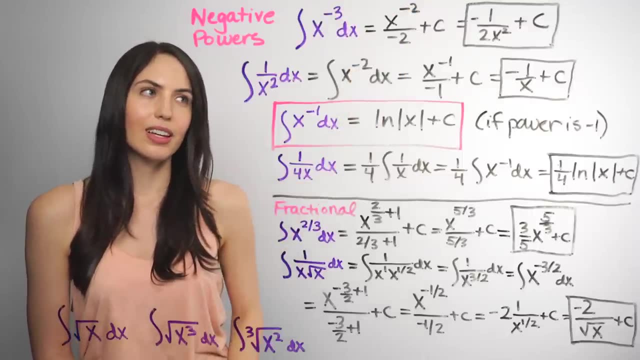 That might be the opposite of what you would think. It's kind of counterintuitive. but increasing that by 1 is going to give you a negative 3 power. So you can make it less negative. so it's negative 2. And I won't waste your time by dwelling 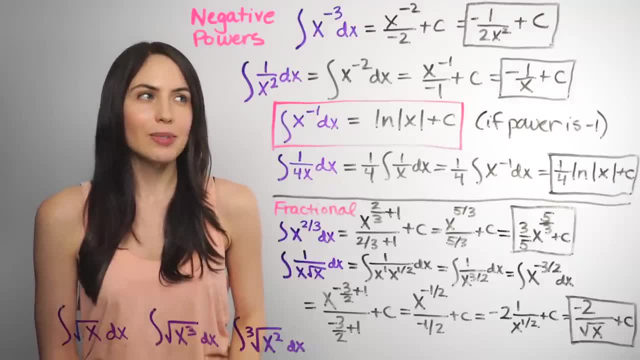 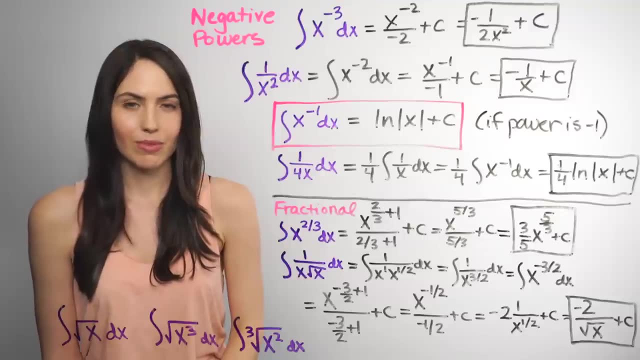 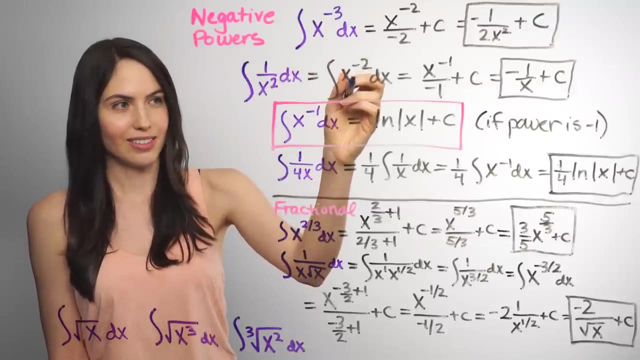 on a lot of algebra here. but a lot of times it's considered simpler to not leave a negative power in your answer, because why not Here? same idea. If you can rewrite it as a negative power, do it And you're going to start to see a theme. 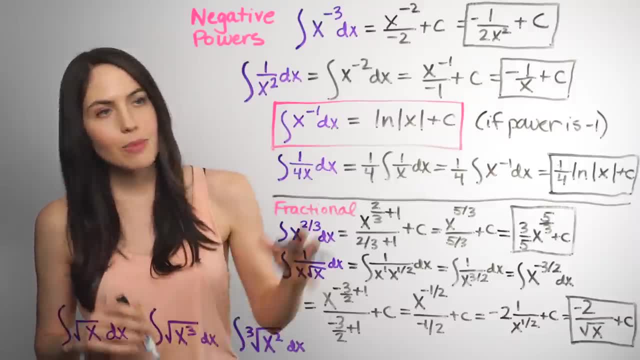 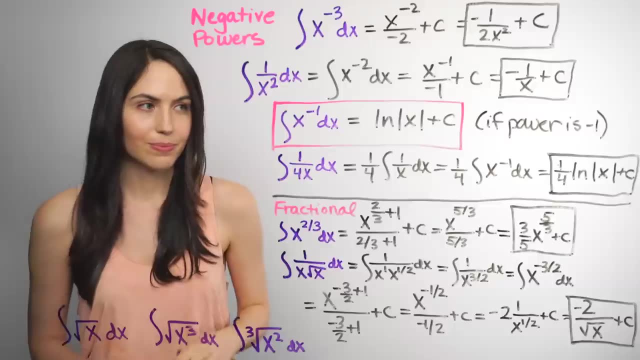 starting here, which is if you can rewrite it as a power up top in the numerator. do that, integrate with the power rule and then simplify. But don't get too comfortable, because I snuck this one in here and maybe you caught it already. 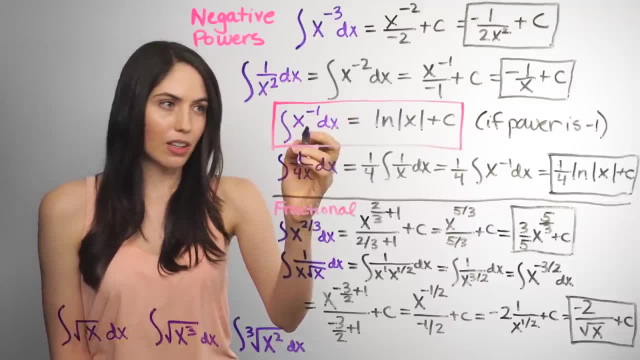 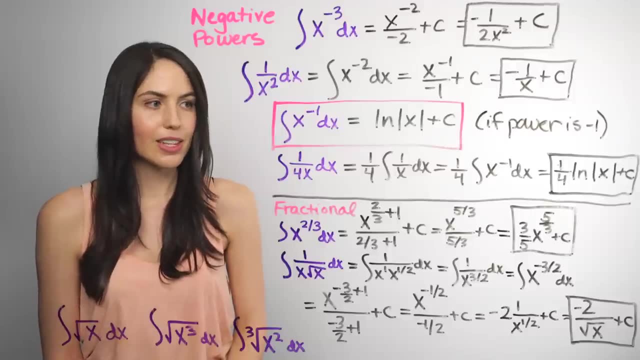 but the power rule is not defined for a negative 1 power. If you look in a table of integrals, it's actually equal to natural log of absolute value of x plus c. So that's what that is And it might actually take this form to. you might see. 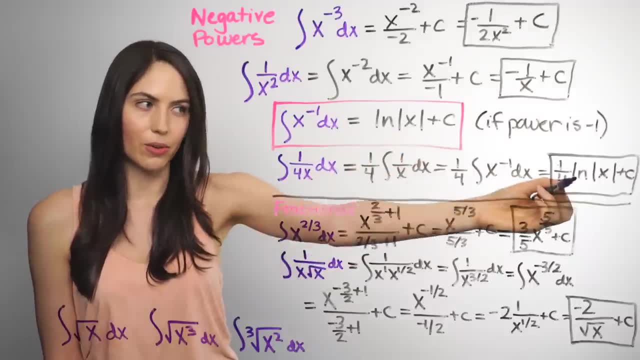 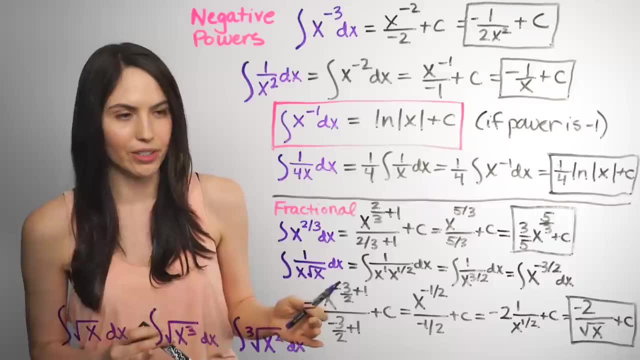 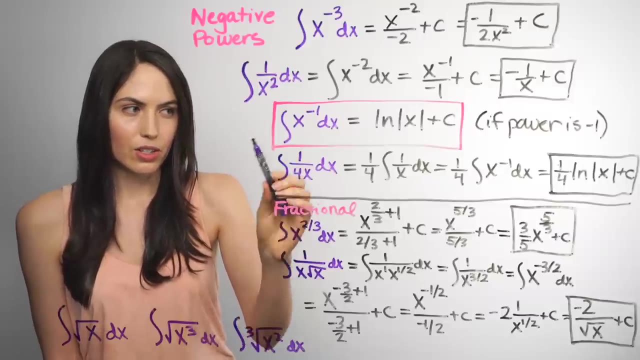 1 over x. that's the same, So that's also natural log of absolute value of x And for this 1. fourth, this is important, if you didn't already know this, for integrals, but any time you can pull out an overall constant out front, do that. 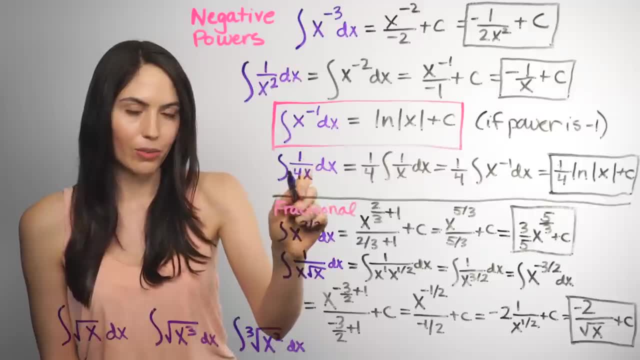 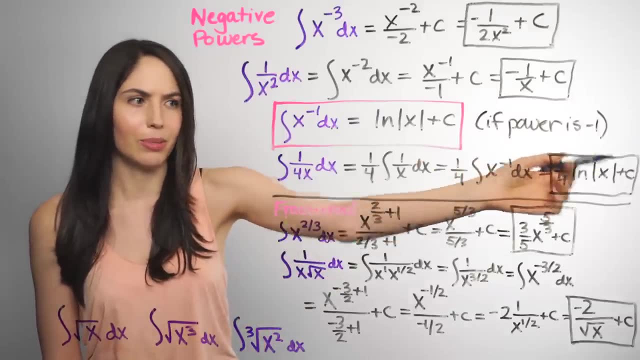 and then integrate the rest. So this 1 fourth can be pulled out front and the rest integrated. If you're wondering why the 1 fourth isn't also on the plus c, thinking it should have been on the c, yeah, maybe, But the thing is we don't. 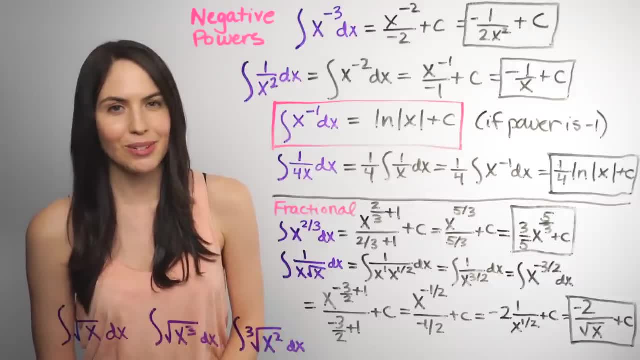 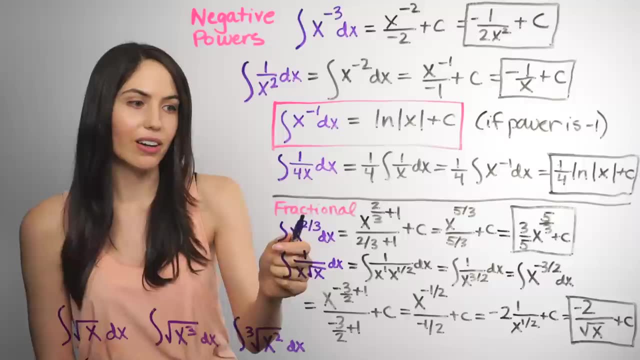 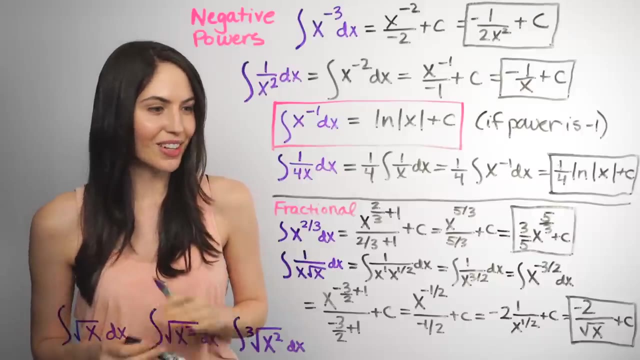 even know what's c. So even if we wrote 1 fourth c, it doesn't really mean much at this point, so we just call it c. still, If you have a fractional power, you can still use the power rule. And again, I'm not going to insult you with a lot of algebra talk. 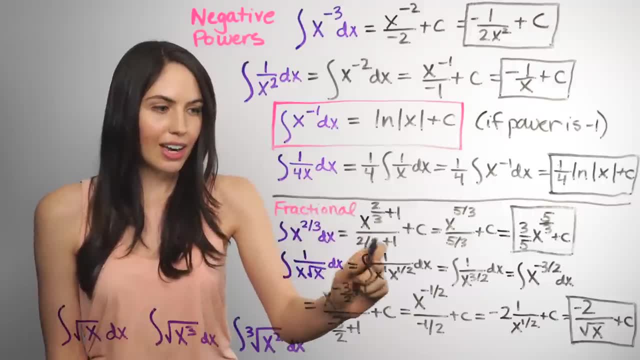 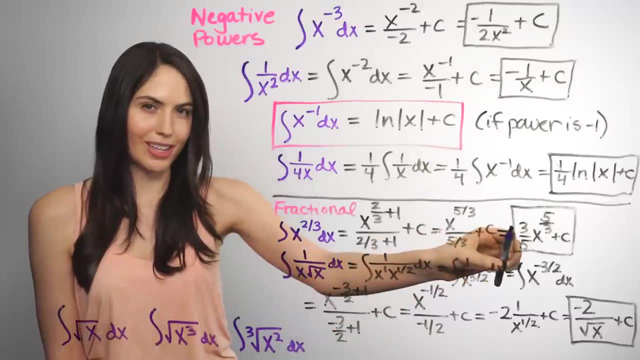 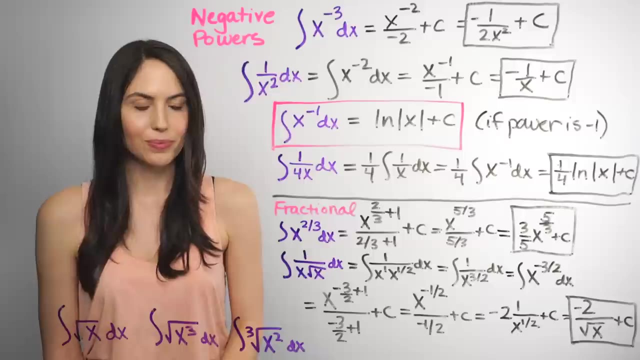 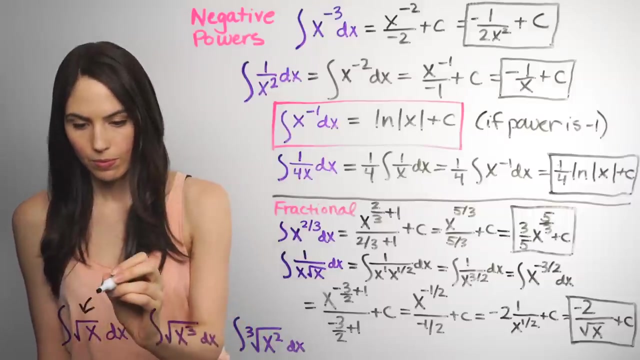 but friendly reminders. adding 1 to a fraction, you get a common denominator. Dividing by a fraction is the same as multiplying by its reciprocal. And what if you have a root in your integral? You might have already guessed, but you want to rewrite it as a power. So square root becomes a 1 half power. 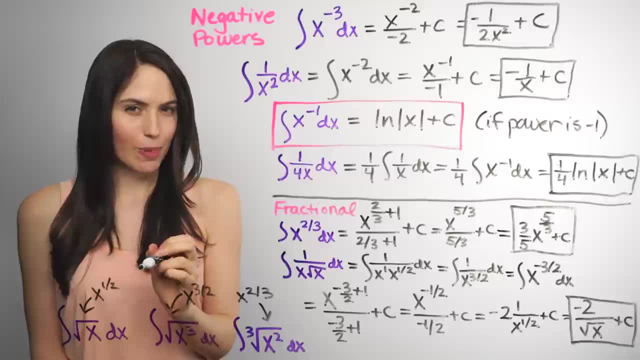 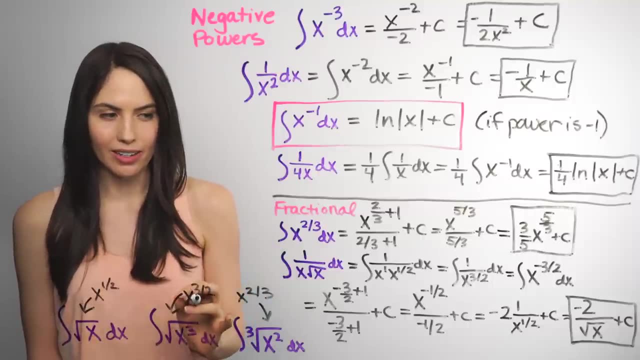 Square root of x cubed is x to the 3 halves power. Cube root of x squared is x to the 2 thirds power, And then you can use the power rule after that, and from there it's the same kind of integration. 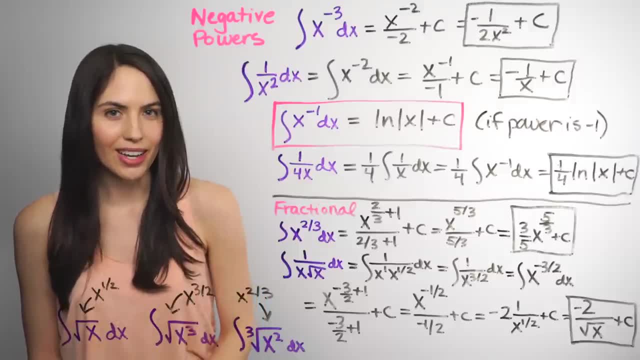 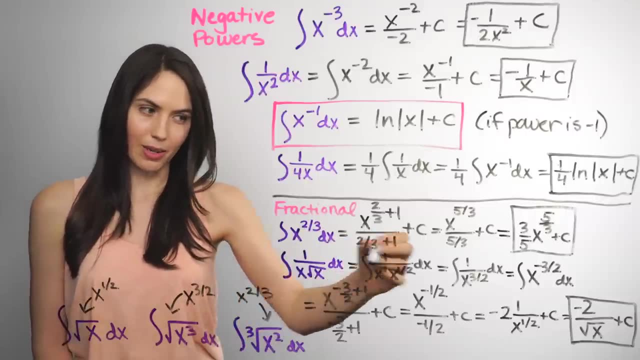 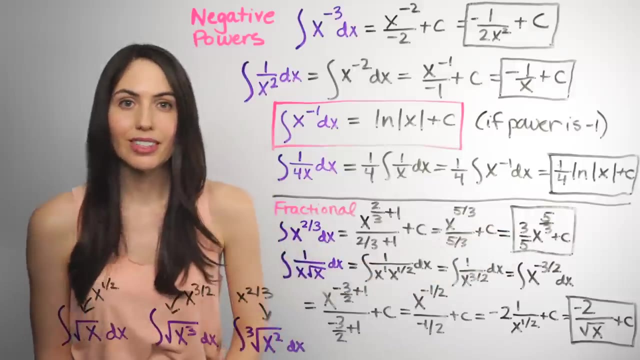 We were doing before. I know you can handle that, but can you handle this? Yes, you can Just rewrite it as powers combine it. Oh look, the power rule: Simplify and that's your answer. You're still alert. That's amazing. 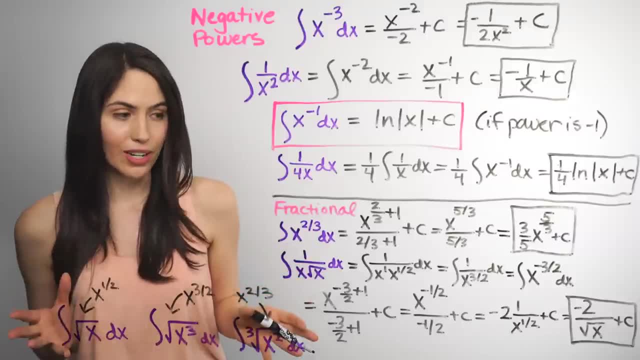 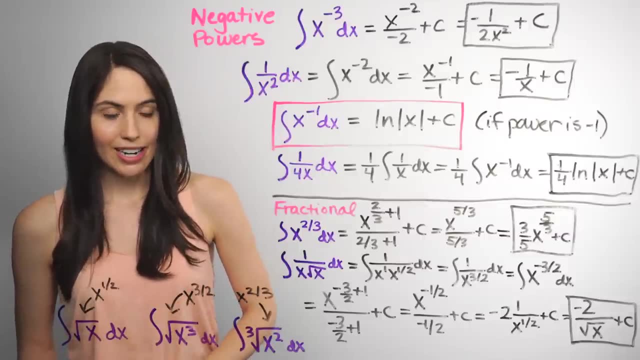 So, no matter what crazy shape it takes when it's thrown at you, the pattern is: rewrite it, integrate and simplify. Rewrite it as a single power and use the power rule. So powers are your friend here, Roots not so much. 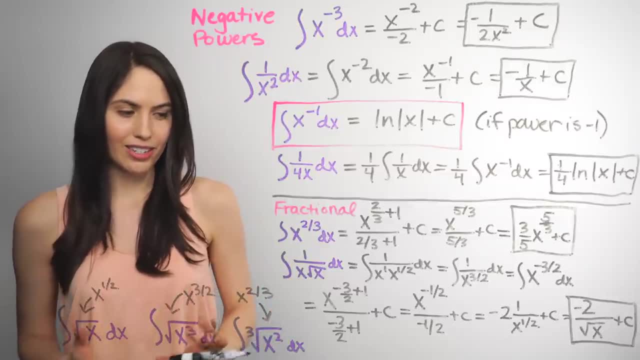 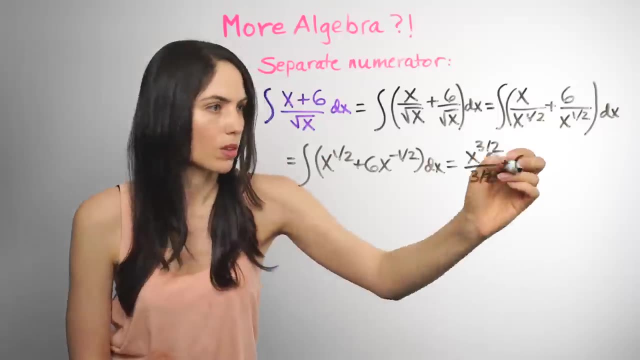 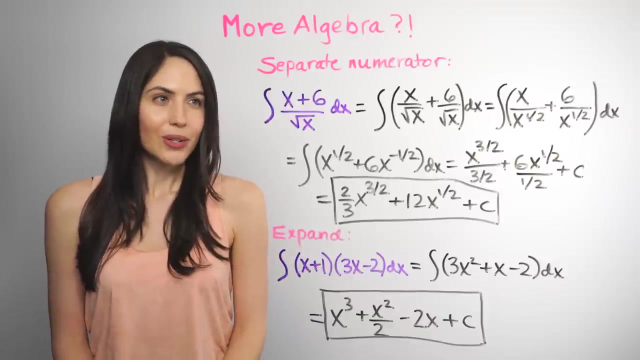 I know this seems like way more algebra than integration, and it is Guess what There's more. So here let's dial up the algebra. What do you do if it does not already look like something you know how to integrate, If you can't tackle it directly? 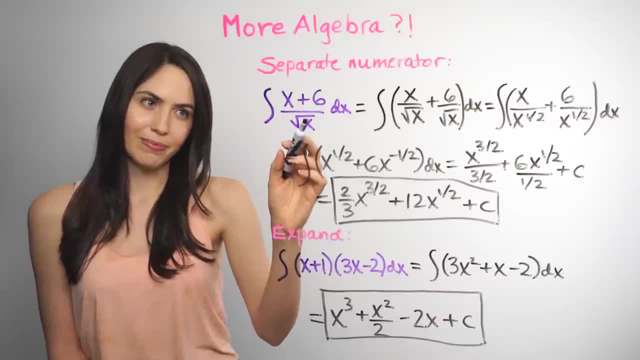 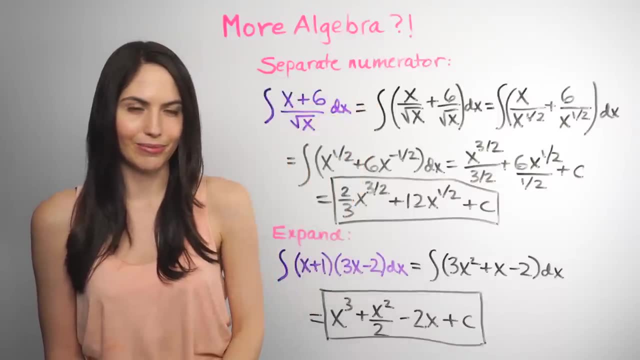 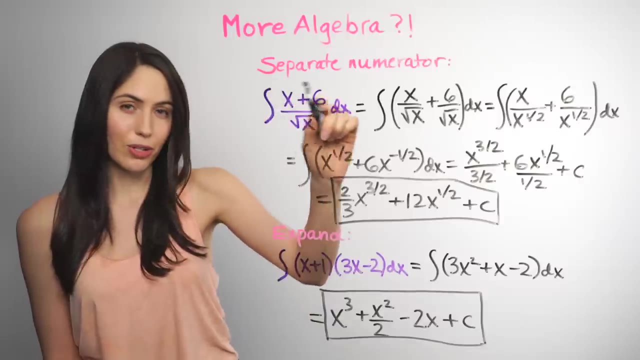 Well, unfortunately there's no quotient rule for integration. And no, you can't just integrate the numerator and denominator separately. That's not? no, that's not a thing. But you can try algebra. Since this is kind of top heavy, a few terms on top. 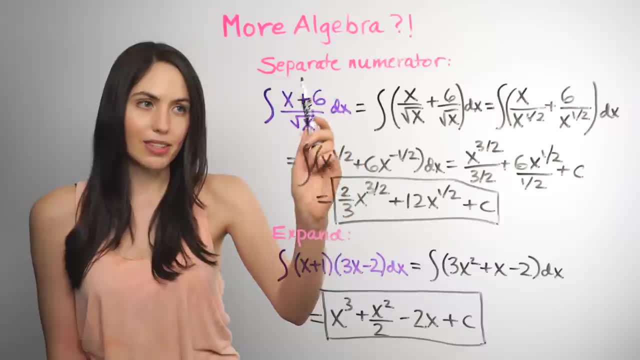 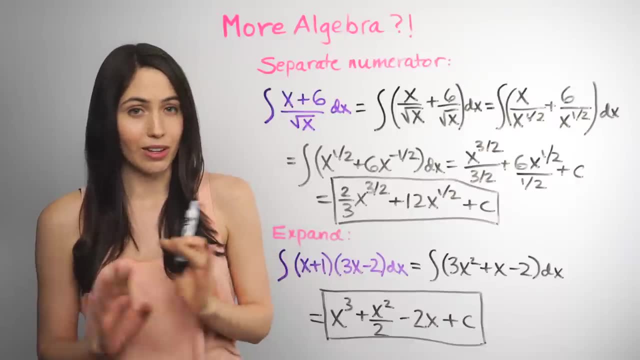 and one on bottom. you can break it into two fractions, separate the numerator, rewrite the roots as powers and simplify. It's not going to hold you hostage with a lot of algebra here, But there's one thing that can be very confusing, which is why would this term 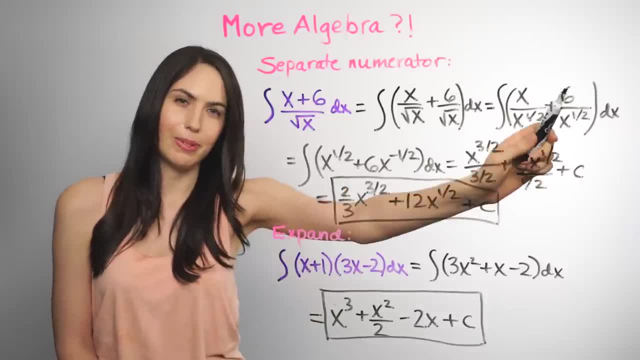 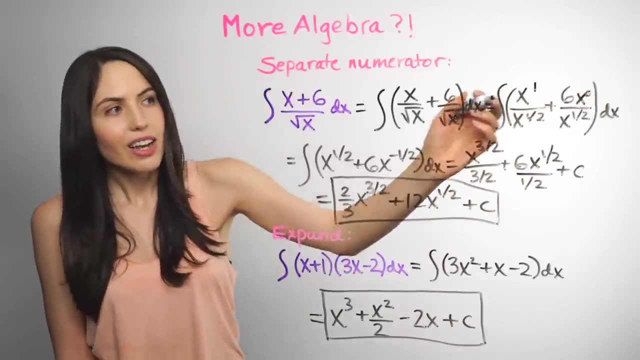 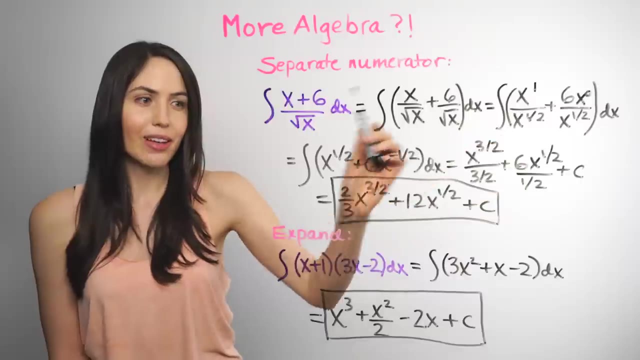 simplify to positive one-half, but this term simplify to negative one-half. Well, if you think of it as x to the first and an invisible x to the zero, subtracting powers would give you one minus a half positive one-half here, but zero minus a half negative one-half there. 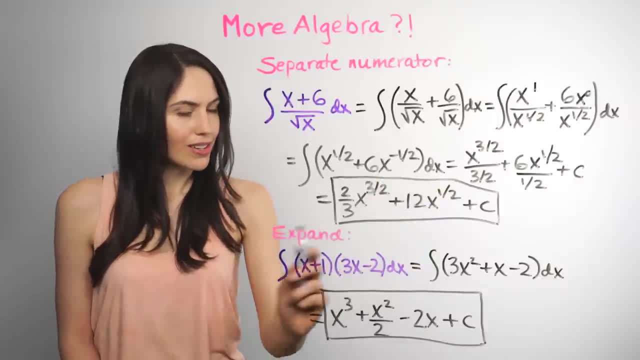 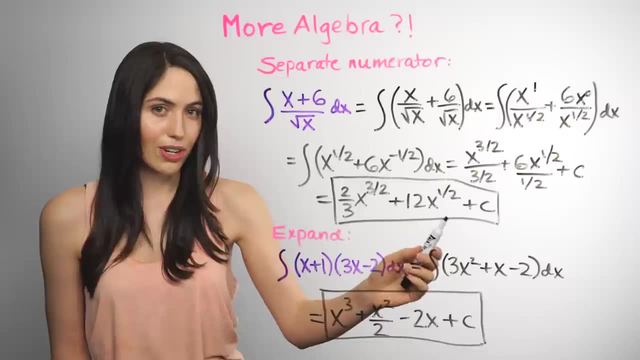 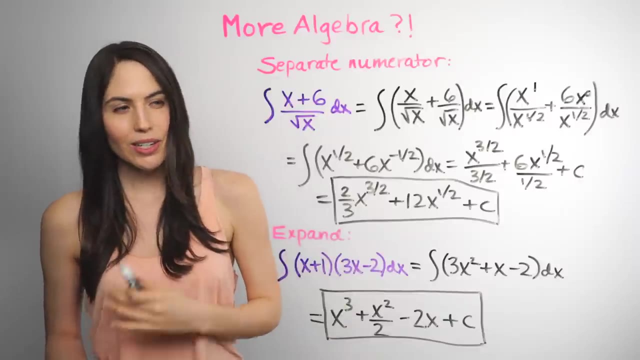 So that's why This one. there's no product rule for integration, but you can multiply it out, distribute it, FOIL it and use the power rule on each term, And that's the answer. So the idea here is always trying to get it into a form that fits a basic integration rule. 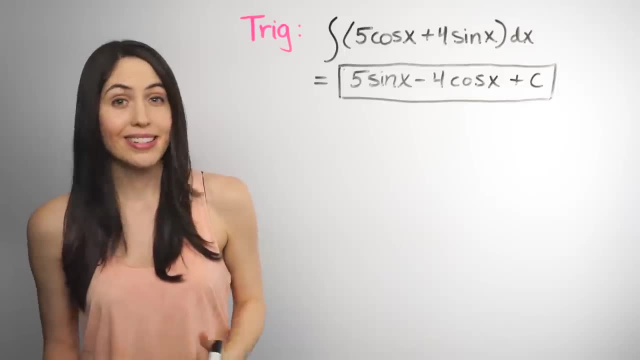 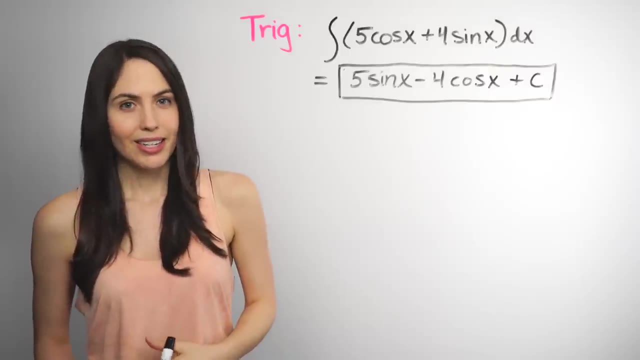 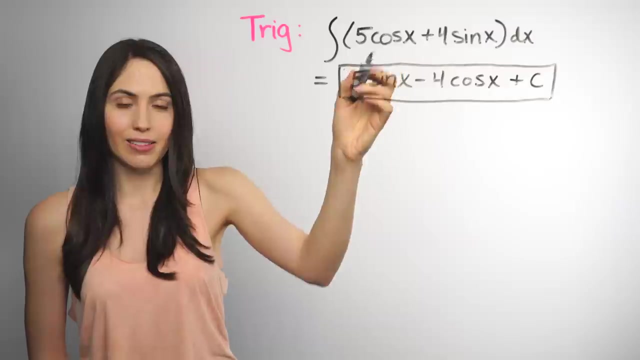 So I keep saying basic integration, The basic integration rules, but so far the only one we've really seen is the power rule. You can find the other ones if you look in a table. If you look up table of integrals, you'll see trig integrals like the integral of cosine is sine. 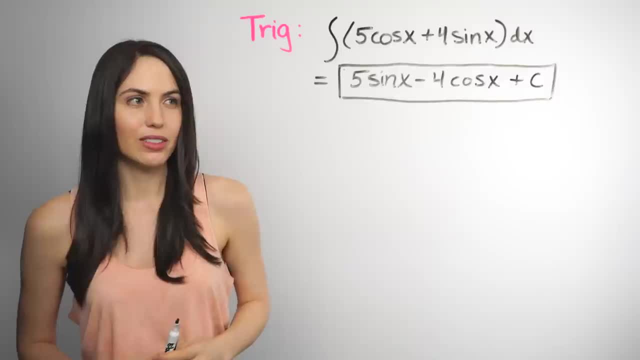 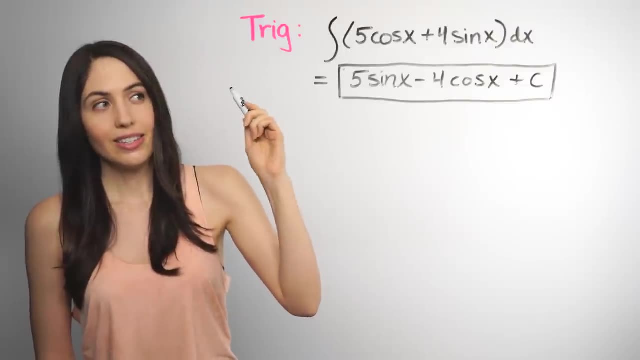 A lot of these are the opposite of derivative rules. hopefully you know. So if the derivative of sine was cosine, then the integral of cosine is sine, And you'll see ones like this: The integral of sine. The integral of sine is negative cosine. 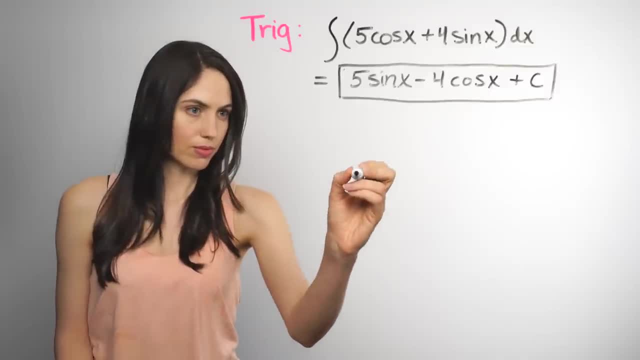 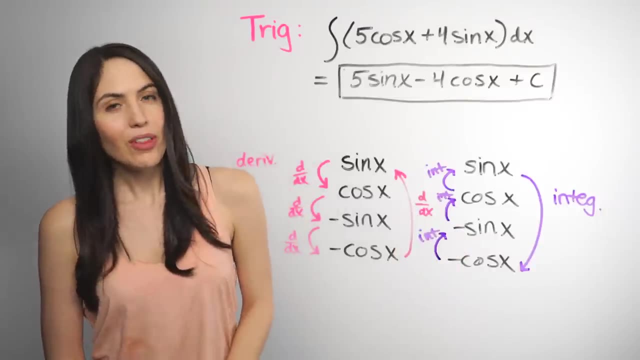 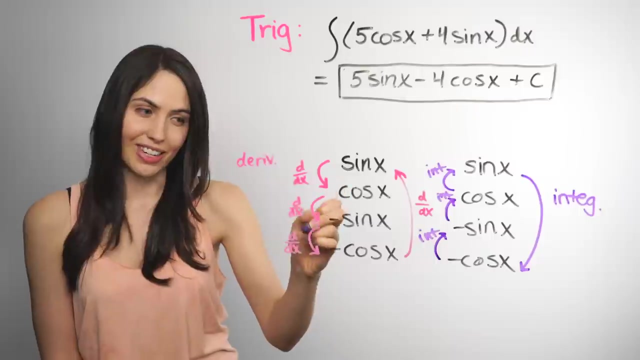 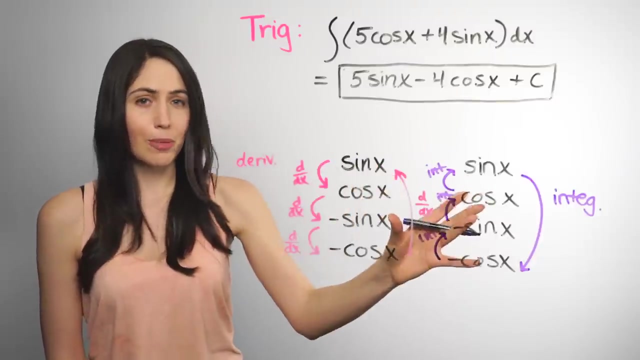 Why is that? Well, remember that the derivative of sine is cosine, The derivative of cosine is negative sine, The derivative of negative sine is negative cosine. And then it circles back: The derivative of negative cosine is sine If integration is the opposite operation. 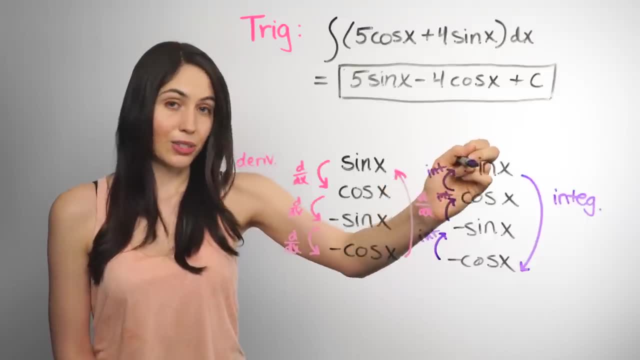 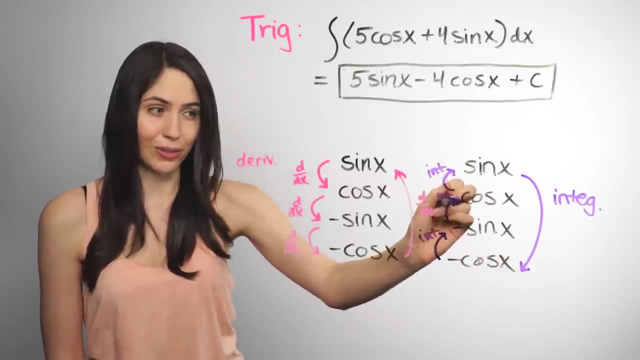 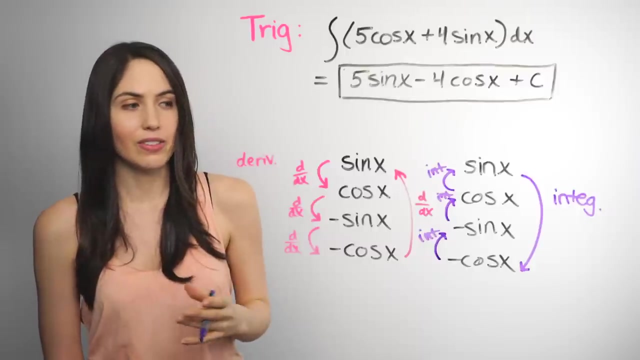 going the other direction. the integral of sine is negative cosine. Integral of that is a negative sine. Integral of that positive cosine, Integral of cosine positive sine. It's cyclical: The sine, cosine, derivatives and antiderivatives repeat in cycles of four. 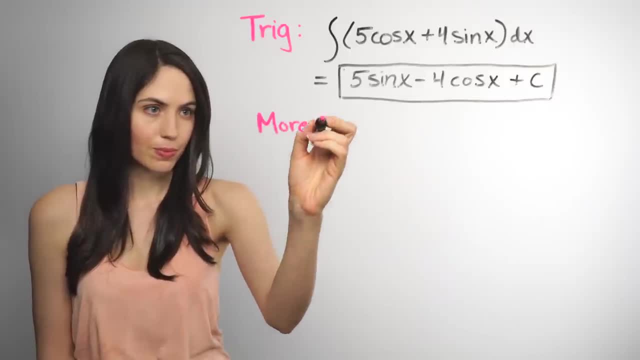 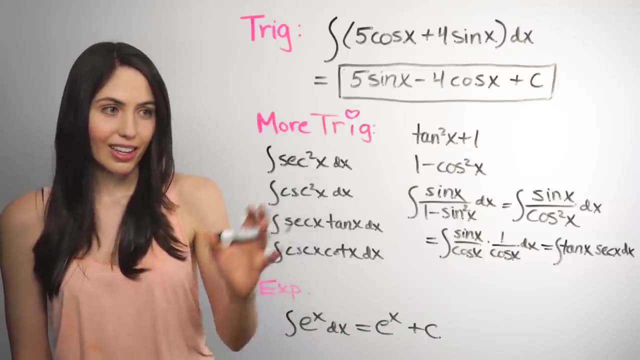 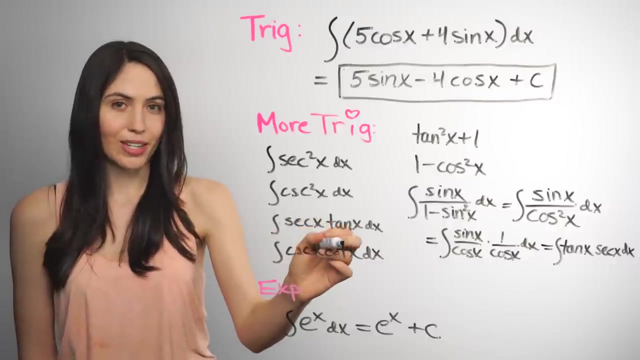 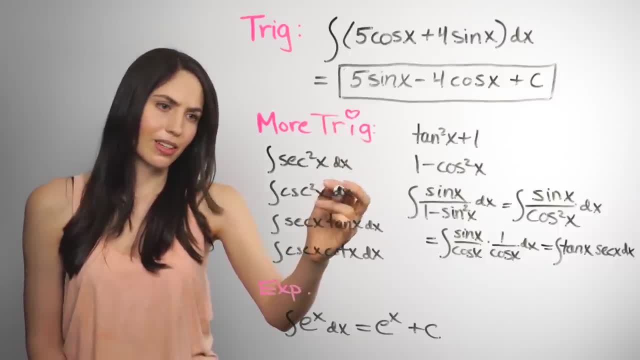 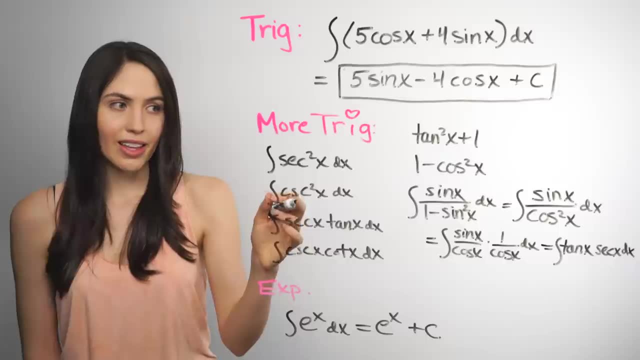 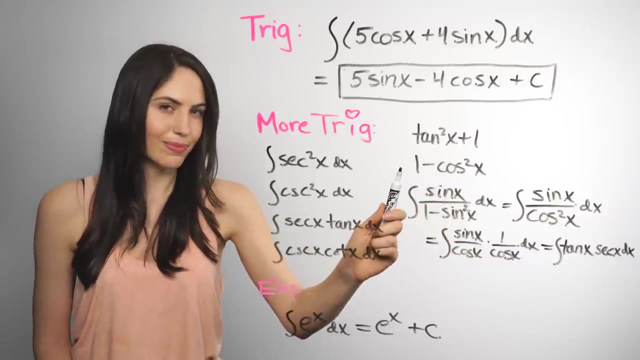 You can look up what they're equal to Like. this is tangent. This equals negative cotangent. This is secant. This is negative cosecant. If you don't see something like this, but you see something like these, you may need trig identities. 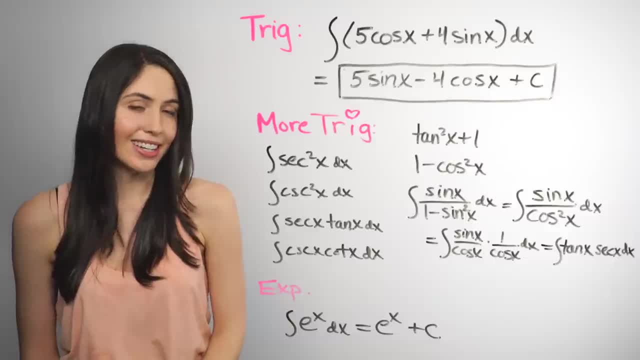 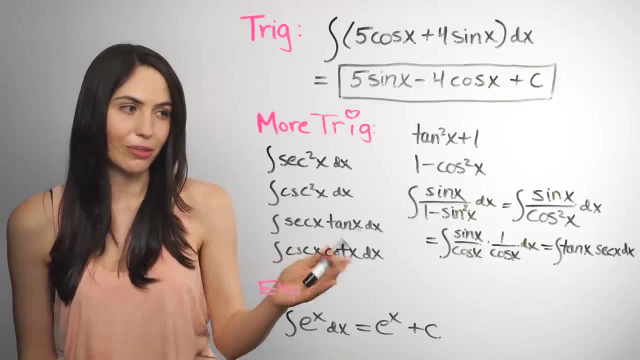 I know some of you have a love-hate relationship with trig identities or a hate-hate relationship. They come up a lot in calculus and here they can help you rewrite the integral in a form that you can integrate. So if you see tangent squared plus one,